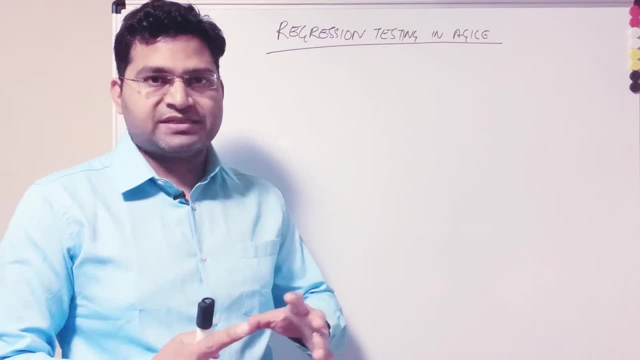 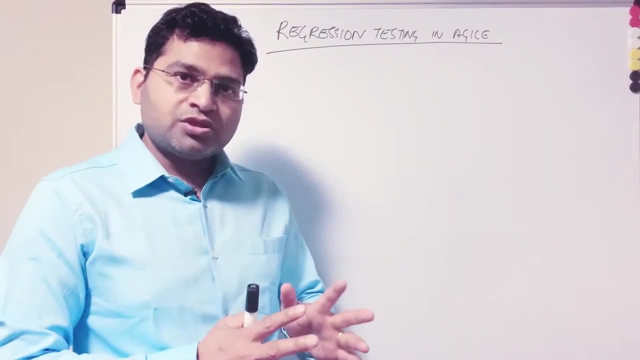 is sort of part of regression testing, but they are not same. So retesting and regression testing are different and I will explain it in the next tutorial. Now, in continuation to what is regression testing, when do you do it? you know we also need to understand what is regression. 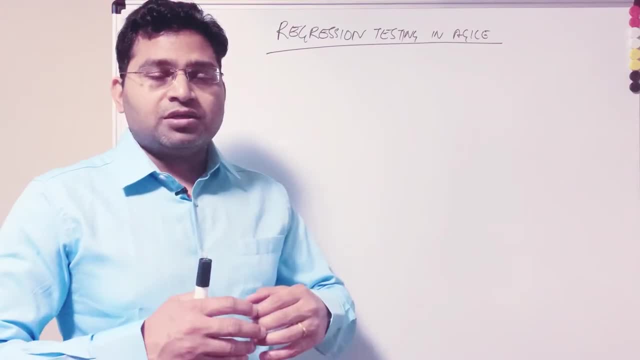 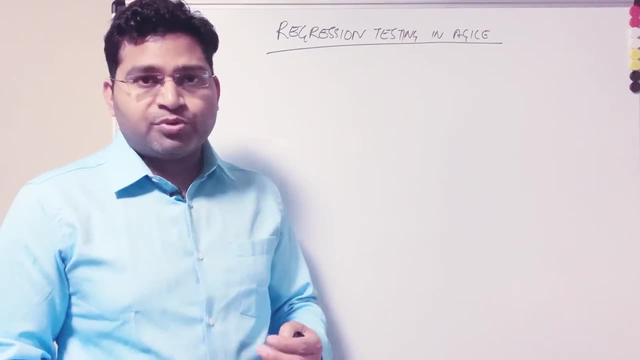 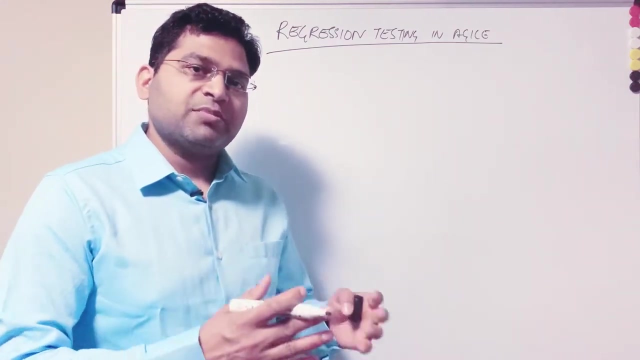 testing in agile or how you need to. basically you know approach regression testing in agile development approach. So if we talk about the agile development approach, say, for example, you are following scrum. So scrum is two to four weeks development cycle. Now in the two to four, 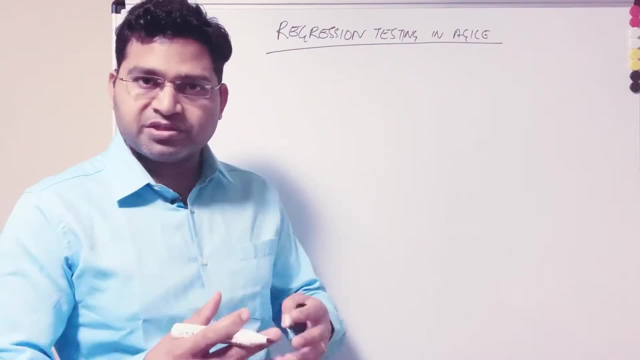 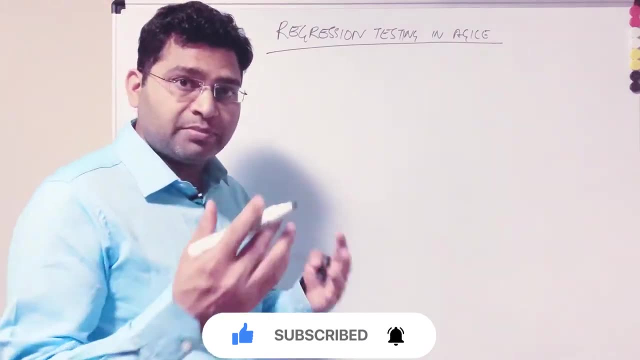 weeks development cycle or iterations, which are also known as sprints. So say, for example, your project follows two week sprint. So what you will have in two week sprint is you will have the sprint backlog. and sprint backlog is nothing but the set of stories or the. 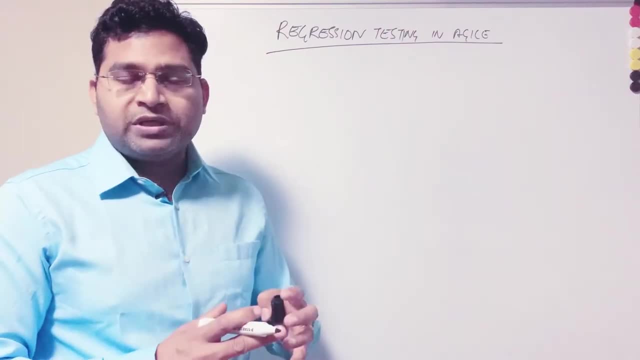 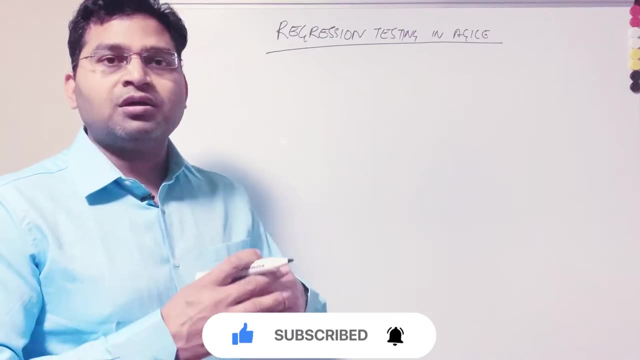 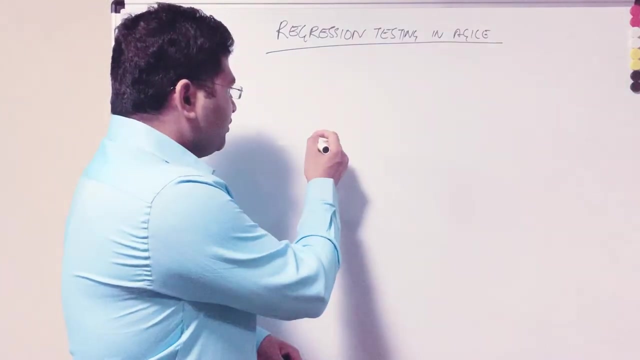 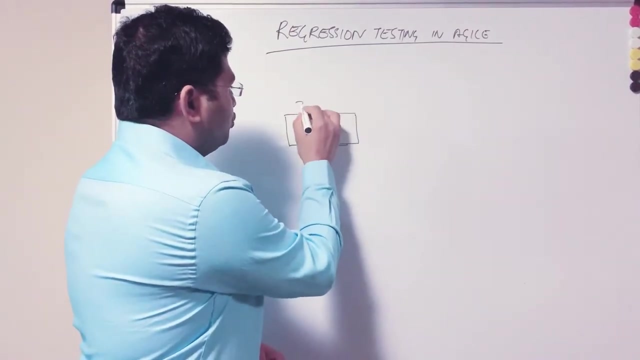 features that you will be, you know, implementing in those two weeks as a team and developing that and basically showcasing or demoing the working software after the two weeks or the sprint gets completed. So basically, sprint one is your first sprint, which is basically, you know, two weeks. 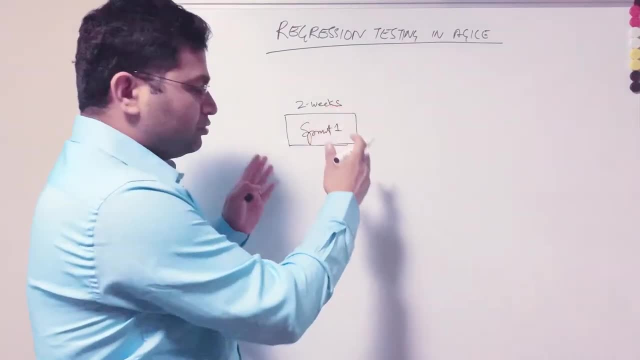 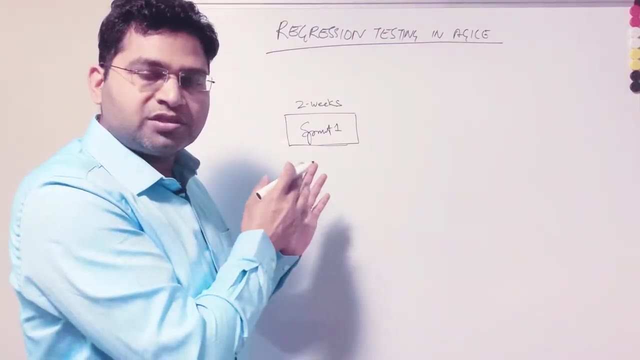 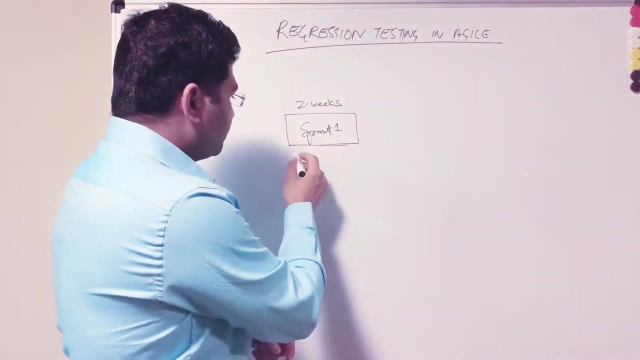 cycle. Okay, So in scrum you will be having, you know, two weeks or whatever cadence that you choose. So if your project has chosen two weeks sprints, then you will be following two week sprints until the completion of the project. So in the two weeks, for example, you have picked, 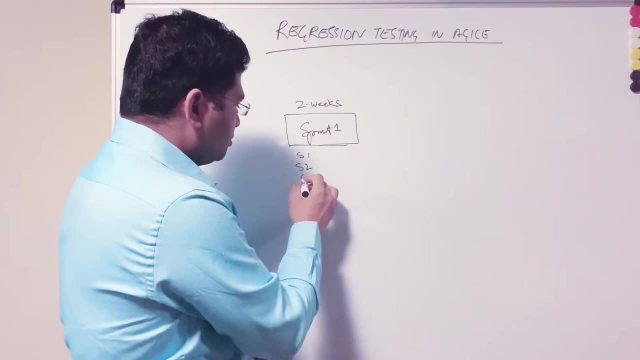 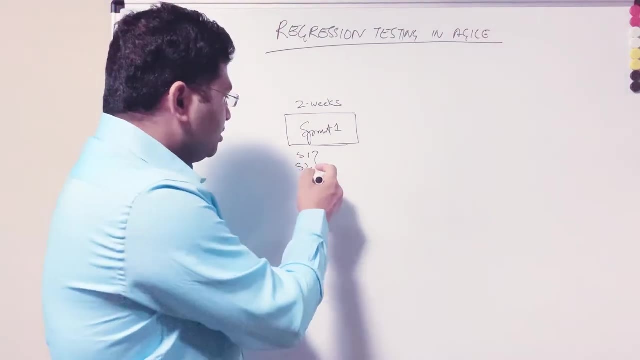 you know four stories, So story one, story two, story three and story four, and stories are nothing but the requirements in the agile project or scrum. So these stories are basically the functionalities that will define, that will have the functionalities and 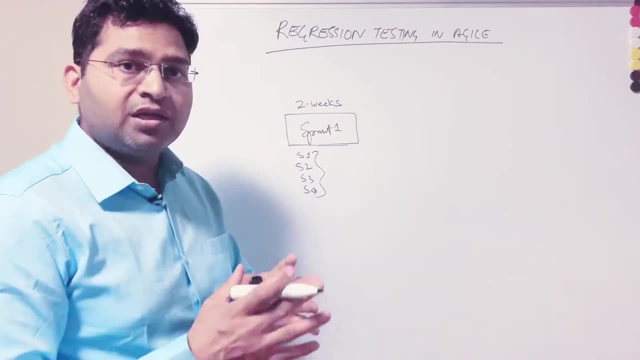 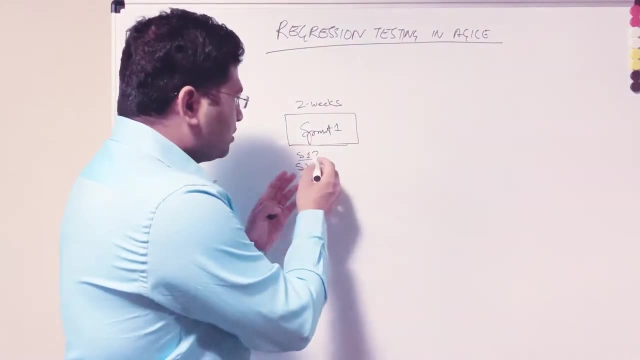 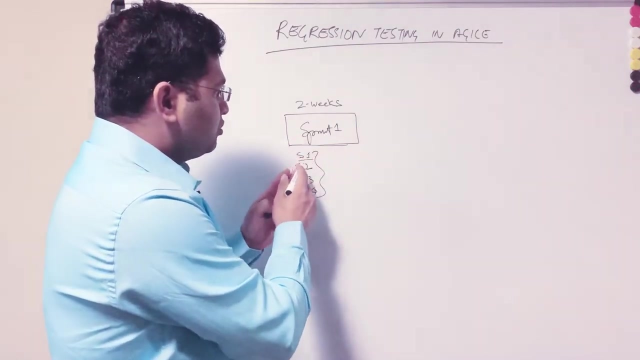 or the requirement and the acceptance criteria which is defined in these stories, And these will be implemented in the sprint right. So developers will start working using these requirements, which are nothing but the stories, user stories, and they'll start developing those user stories. 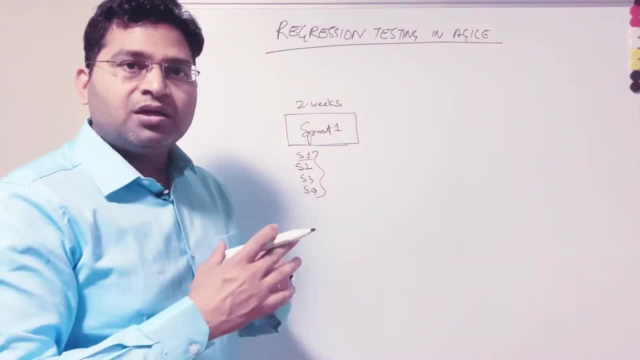 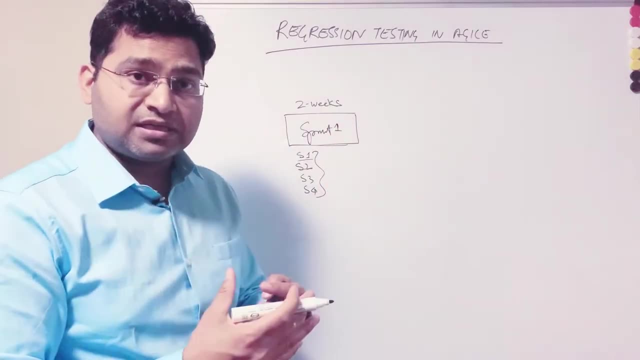 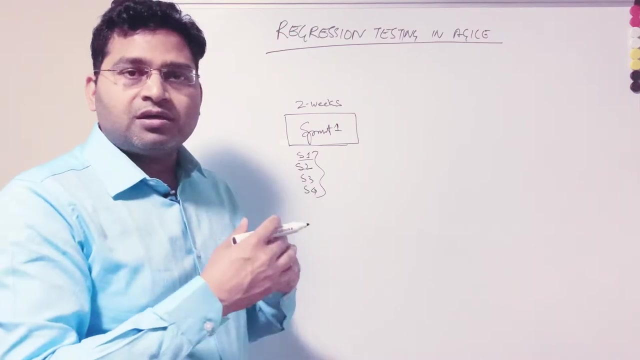 Testers will collaborate With developers, BAs, and they'll start, you know, documenting or writing the test cases And, as soon as the functionalities are available, testers will start testing the stories and ensure that the acceptance criteria that is met in these stories is, as expected, right. So when we talk about 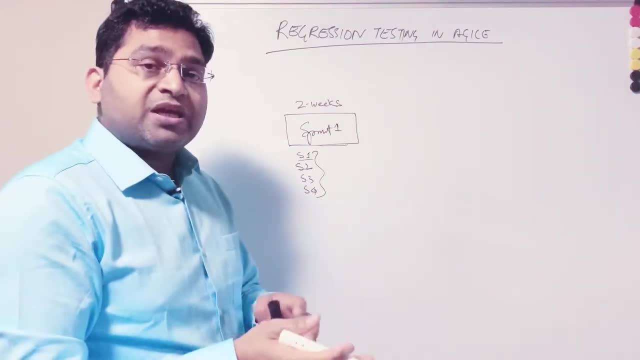 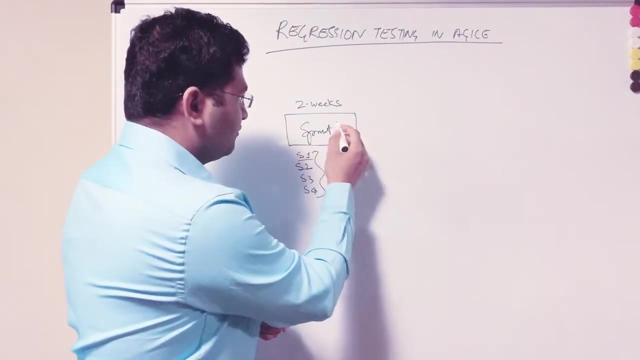 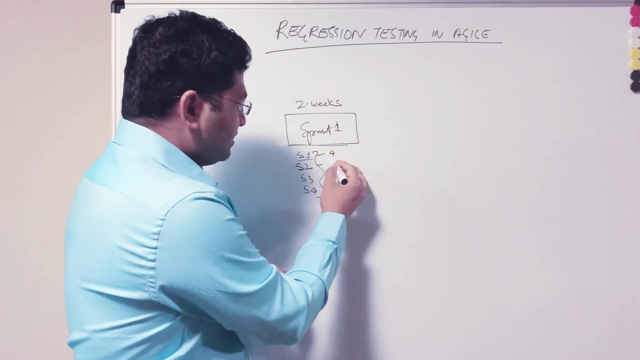 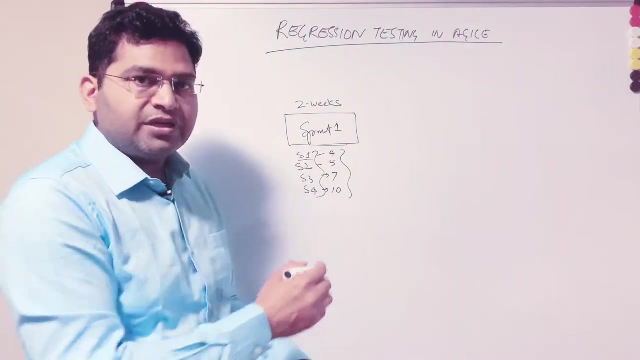 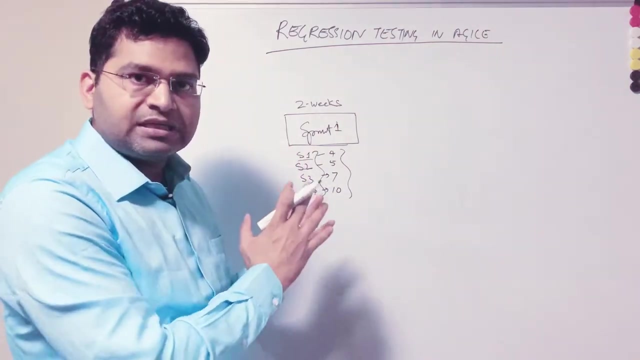 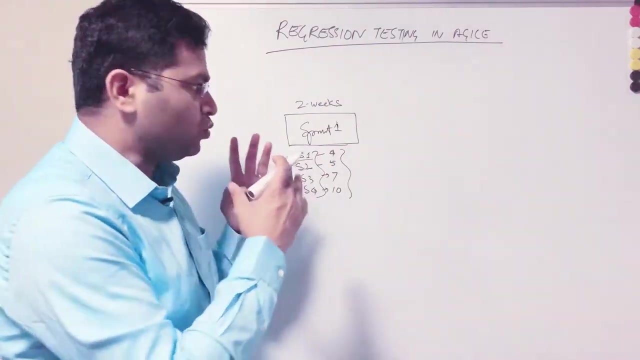 regression testing in agile. how it is, it becomes challenging in agile If you cater for the manual regression testing. we'll understand that. So let's say, for example, this is the first sprint and you have four stories and each story has say: for example, this story has four test cases, this has five, this has, you know, seven and this has 10 test cases, right So these are the test cases that you have written for these four user stories to verify that the functionality that is defined in these user stories is as expected. right Now, this is the number of test cases that you have written and executed in sprint one. 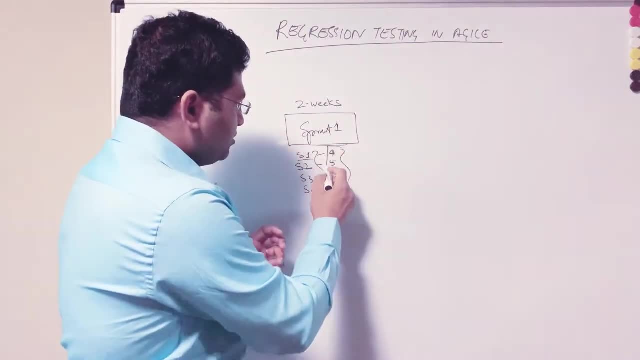 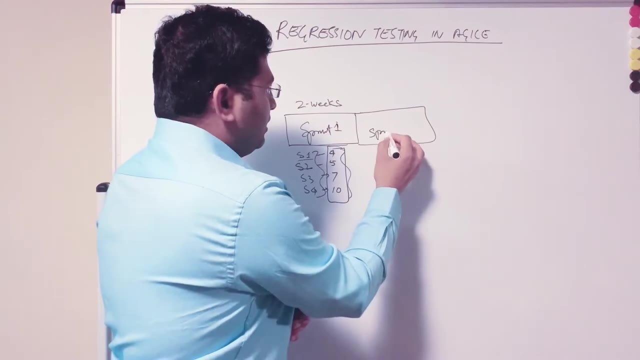 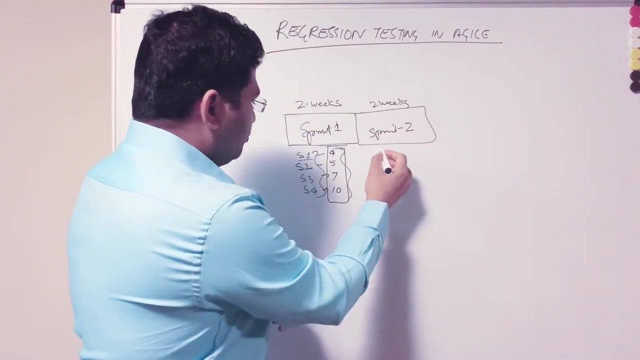 Now, once sprint one got over, say, for example, here you have executed all of these. you know manually right. So there will be another next sprint, which is sprint two, And in sprint two, which is again next two weeks cycle, and in sprint two you will get another user requirements. 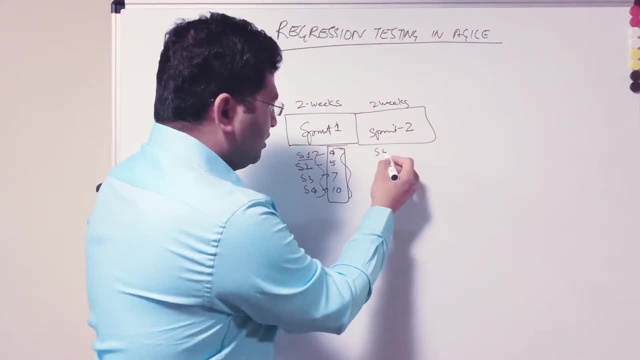 right. So another user story is based on the priority. say for example, five, six, seven, eight, right, So four stories again. or maybe you know like nine stories, depending on the priority. So five, six, seven, eight, right, So four stories again. or maybe you know. 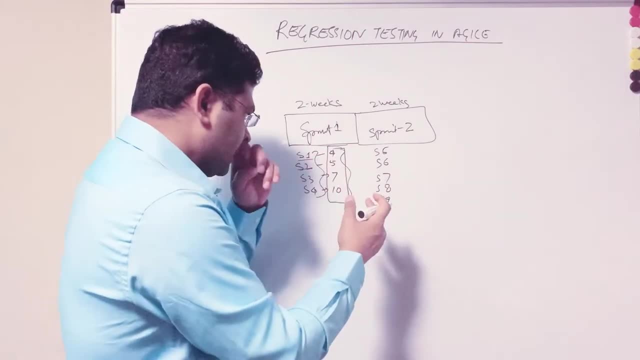 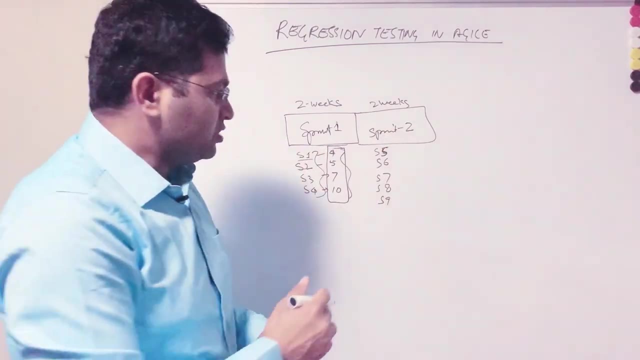 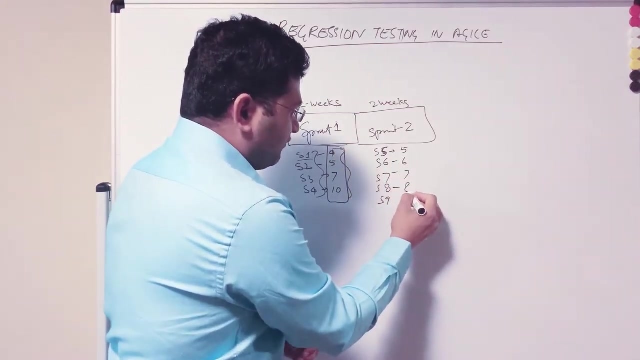 like nine stories on. you know capacity of the team and the size of the stories. so in the next print now you have five more user stories to actually test and you are documenting the test cases for these user stories. okay, so you have couple of test cases written for these user stories and now these: 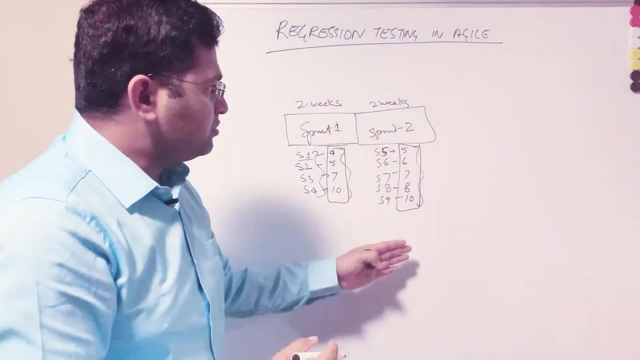 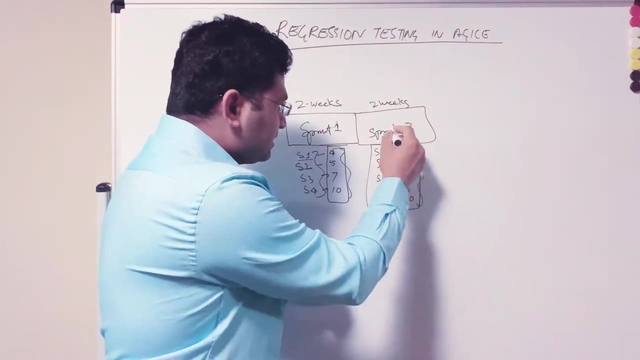 are the number of test cases that you have written for these user stories for sprint 2.. so you will be doing the progression testing, which is functional testing of these user stories, in the second sprint as well as because in the second sprint the code that has been written. 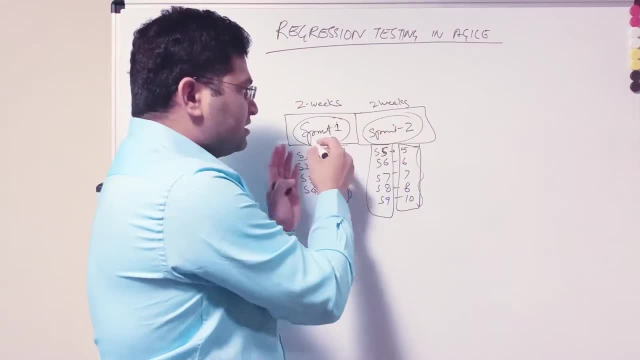 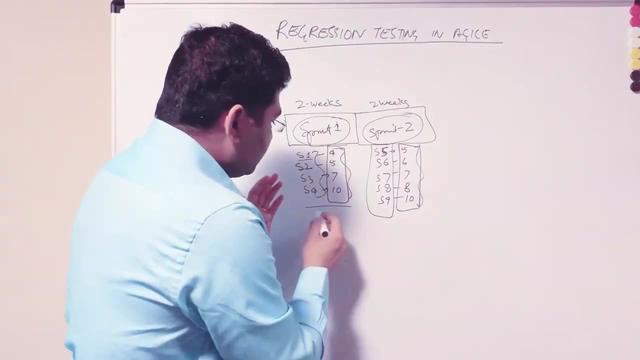 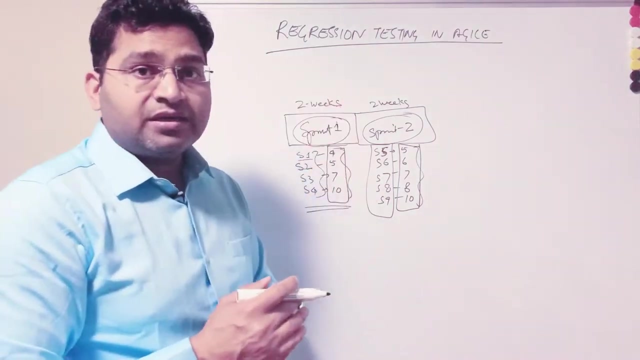 in the first print there will be new addition to the code that is written in sprint one from sprint 2 as well. then you need to ensure that the existing functionality that was working in sprint one hasn't broken right. so that is what a regression testing is. 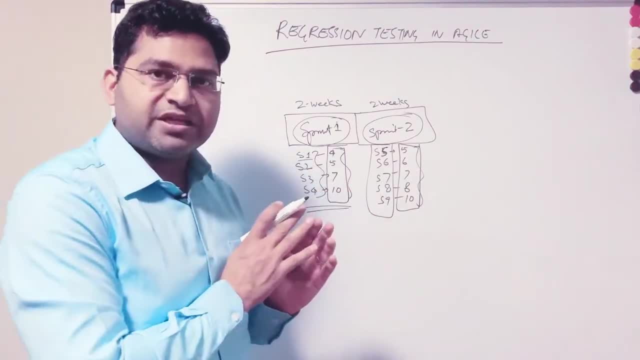 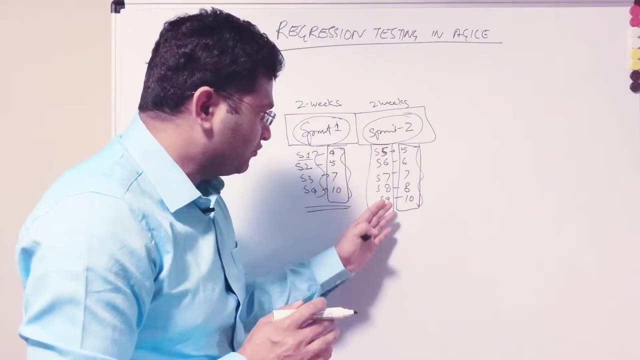 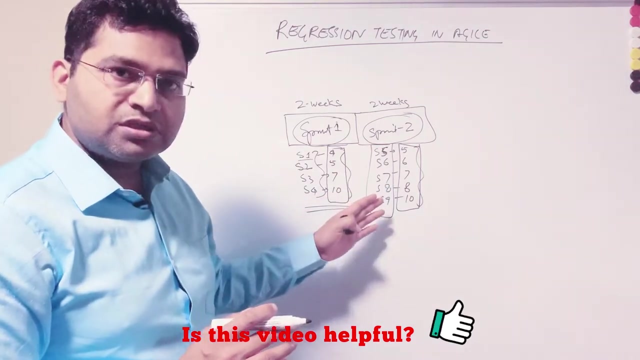 to ensure, Ensure that any existing functionality of the application that has already been working prior to the new implementation, be it addition of the new functionality, which is, in this case, you know, addition of the new functionality that are part of the user stories. 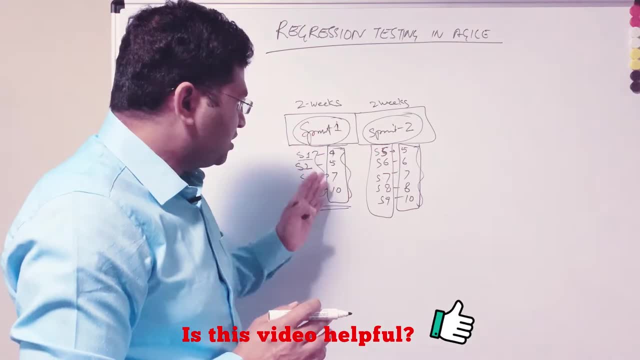 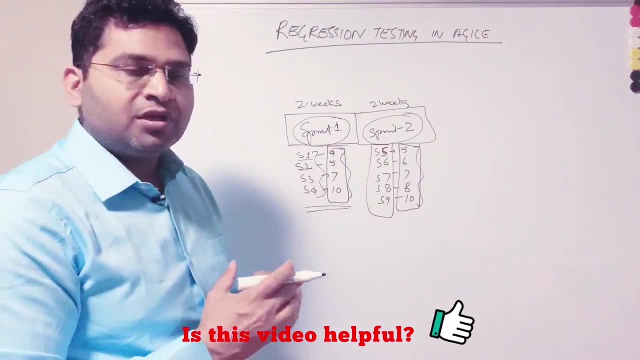 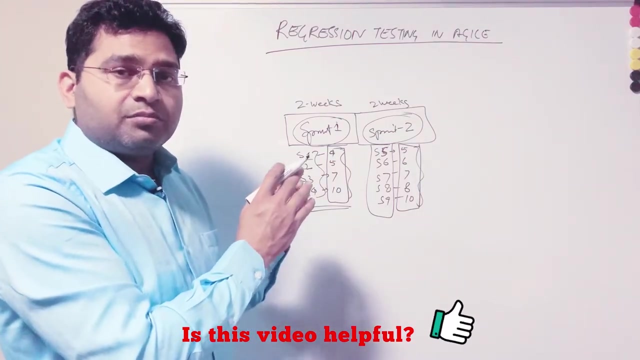 Or if say, for example, there was a defect that you raised in sprint one and that got fixed, so you re-executed So any updates that happen. you need to re-execute the existing functionality or a subset of existing functionality based on the addition, whatever updation has been done, and ensure that existing functionality works. 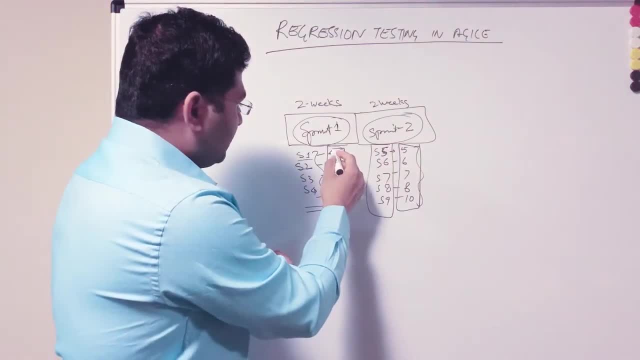 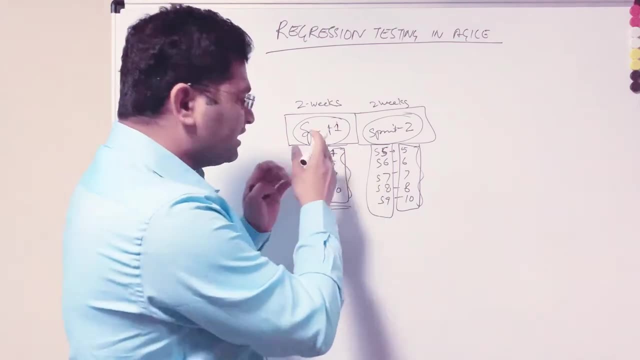 So, in this particular case, what you need to do is you need to either pick all of the test cases that you have picked in sprint one and re-execute in sprint two to ensure that everything that was passed in sprint one is still working right. 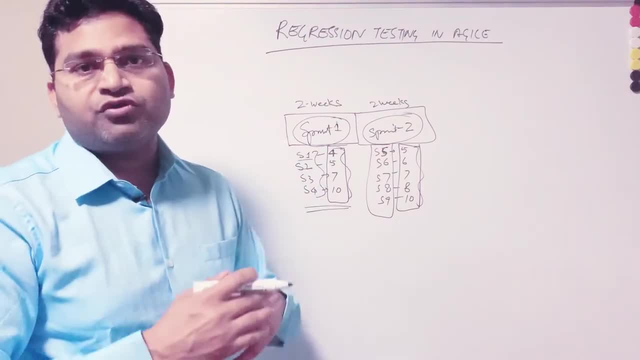 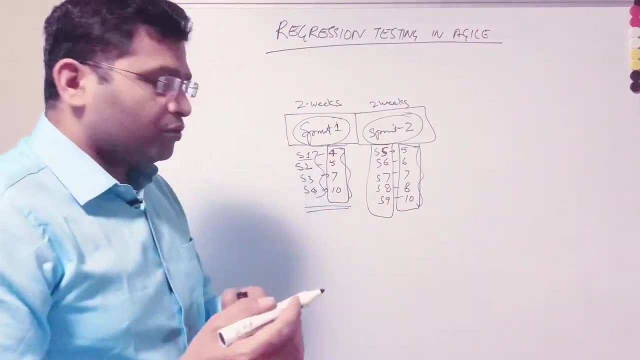 But that is really, really not feasible in agile project. if you are doing the manual testing or even if you are doing the automation testing, So what you do in agile projects- you know the reason for that is why it is not feasible. So, for example, there is another sprint three. 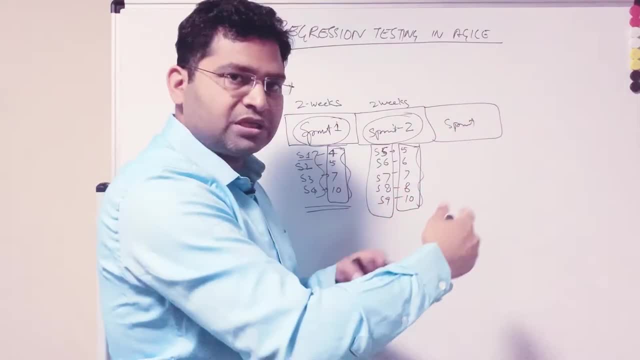 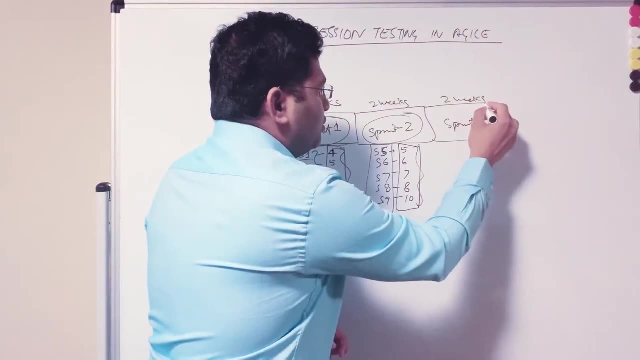 OK, so there will be like 10,, 15,, 20 sprints, you know, until you release the software. It depends how big your project is. So in sprint three, which is another two weeks, you will be having some more stories. 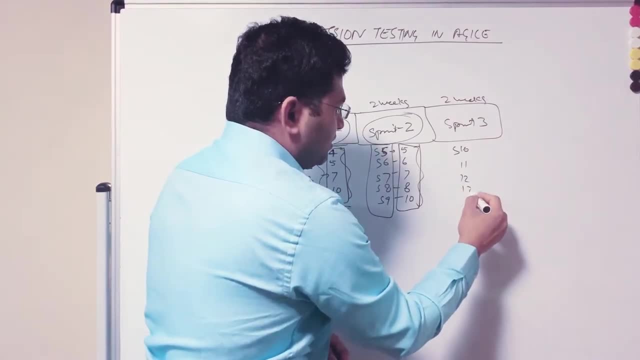 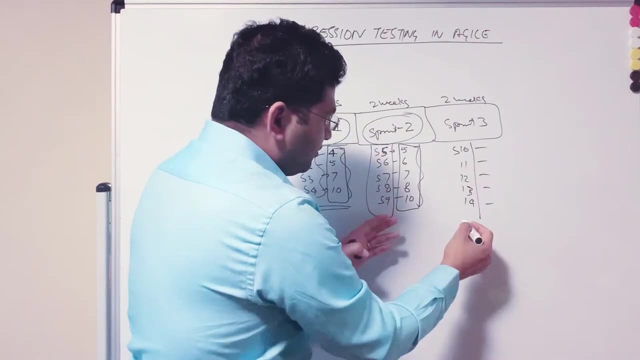 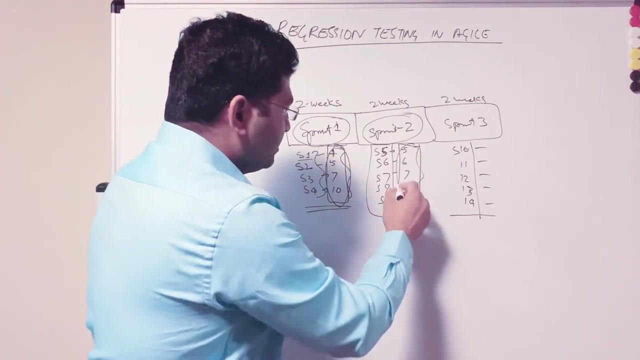 Right, So 10,, 11,, 12,, 13,, 14.. So, like four, five more stories There will be, you know, new test cases. And then here, if you want to execute the overall test cases or regression test cases, you have to execute these plus these and then plus the functional test cases that you write in sprint three. So, with each and every upcoming sprint, your number of test cases that need to be executed as part of the regression. So- And that is not possible with the size of team that you will be having- You can't keep adding new members or new addition to your team in each sprint. 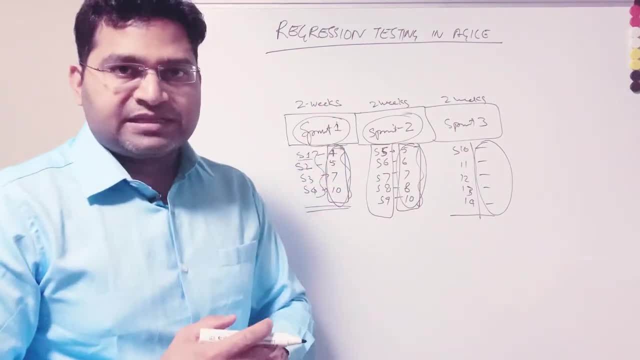 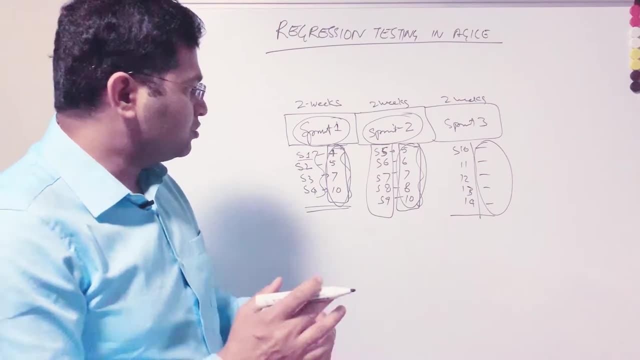 So this is the biggest challenge in the agile testing approach Right now. how you can tackle it is basically through automation, Right? So the first thing is to basically if say, for example, in this particular sprint you have a couple of test cases, 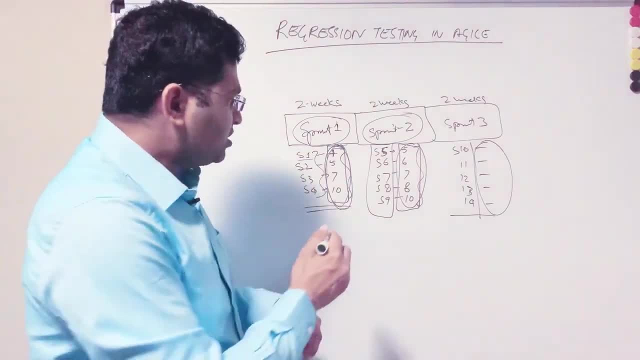 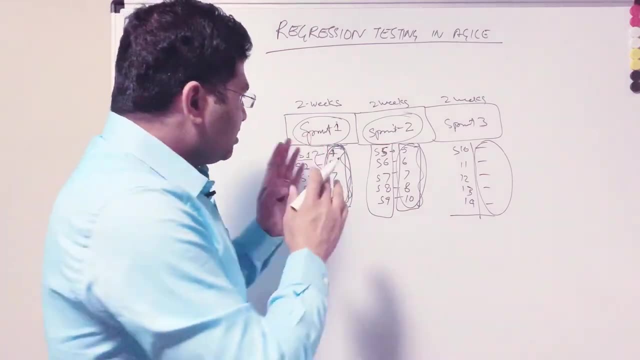 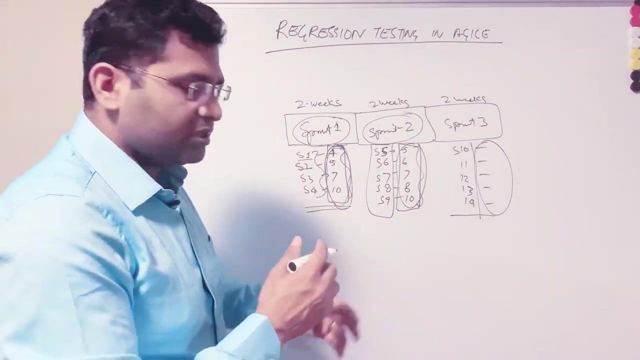 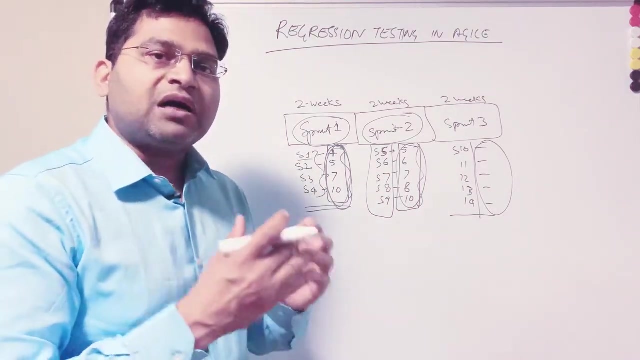 So you can target, as part of the automation, you automate the regression test cases that you have identified from this list. So, in the sprint one, as you do the progression test cases, or the test cases that have been part of these stories, you also keep marking them, which of them are very important and need to be part of the regression suite. 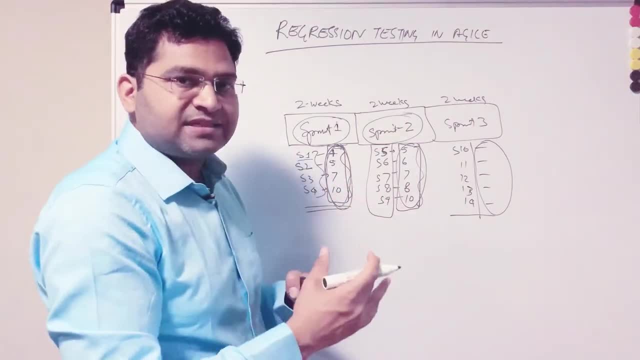 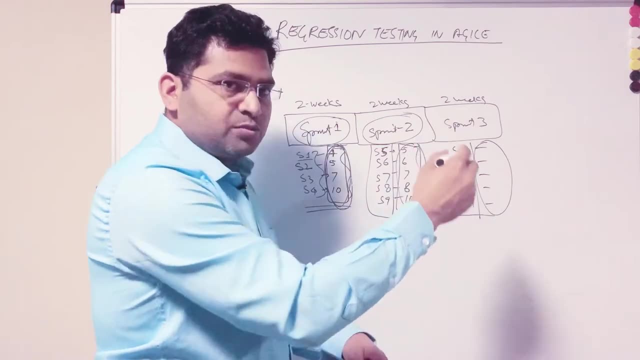 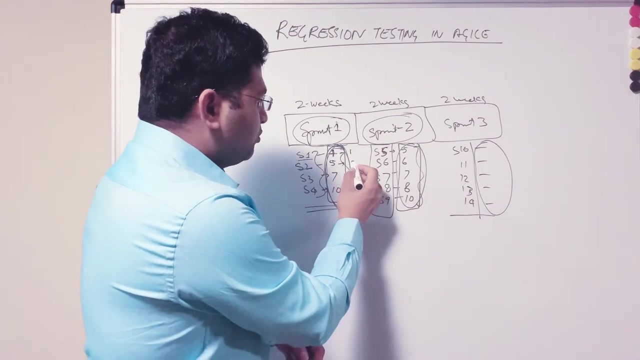 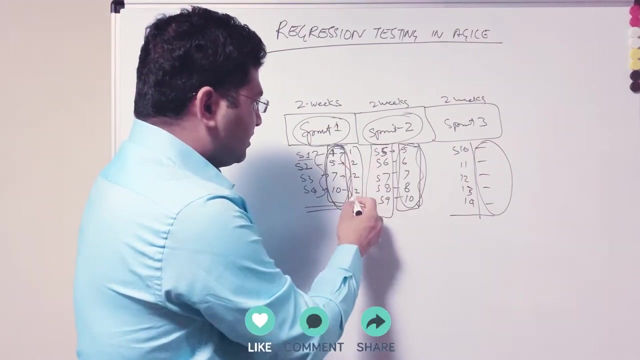 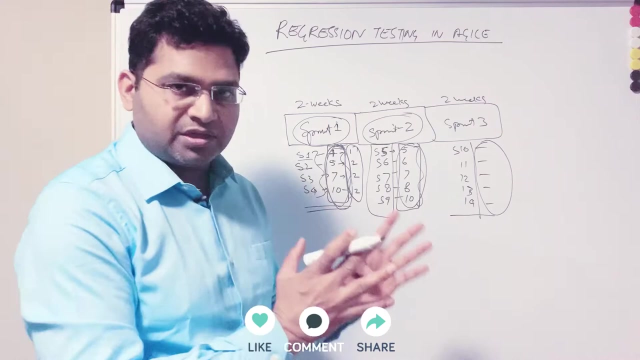 So you, in the tool itself, you mark those test cases As I as a regression, so that your regression test suite gets built as you progress with within the sprint. along with that, you need to say, for example, out of these four test cases, you mark one as a regression candidate, you mark two out of these five as a regression candidate, two out of these seven, and then two out of these 10 as a regression candidate. you should not try to include all of the test cases that you have tested as part of the functional testing as the regression test suite. 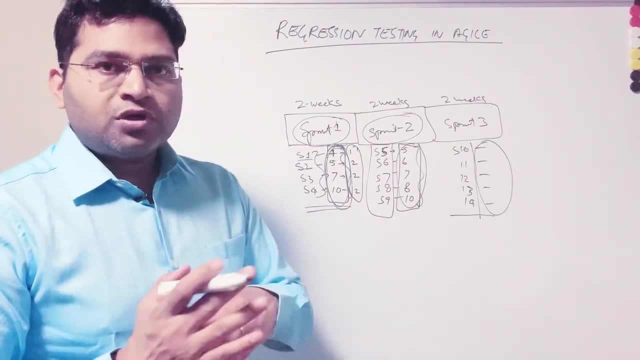 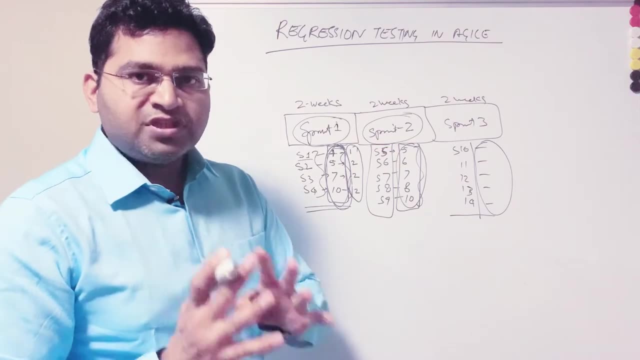 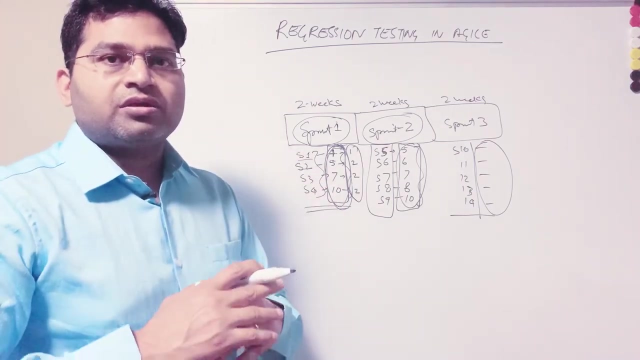 If you're doing that, then you are Basically, you know, not segregating what is really important and what is less important in the project. and in a project or in a, in the features, everything can't be important, right, So it has to be prioritized based on the highest priority, or the highest usage and the low usage and the low priority. 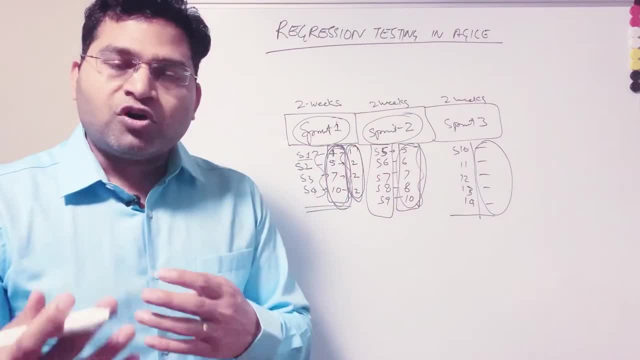 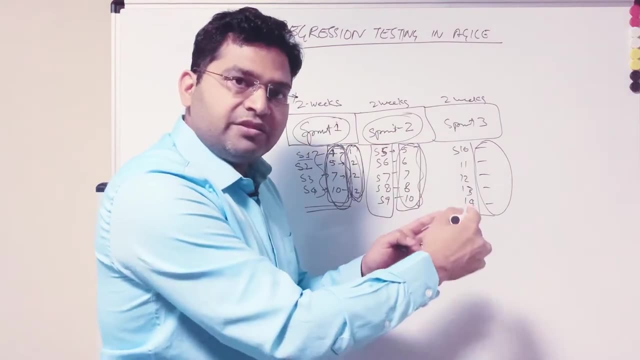 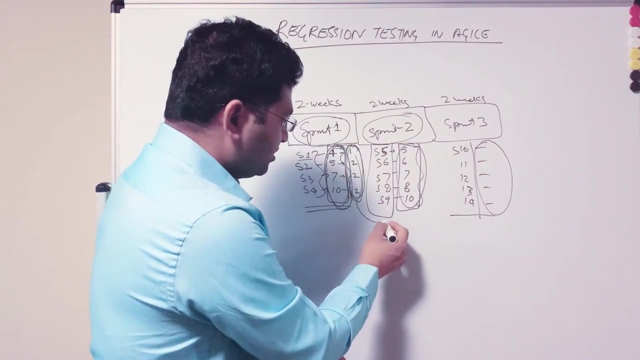 So, based on that, you basically come up with the test cases that will form your regression test suite, right? And these test suite you try to automate as you progress along In the sprint in the agile project, right? So say, for example, now I have, you know, seven test cases in the next sprint. 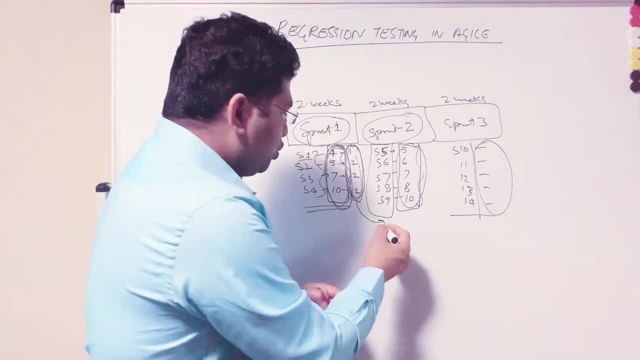 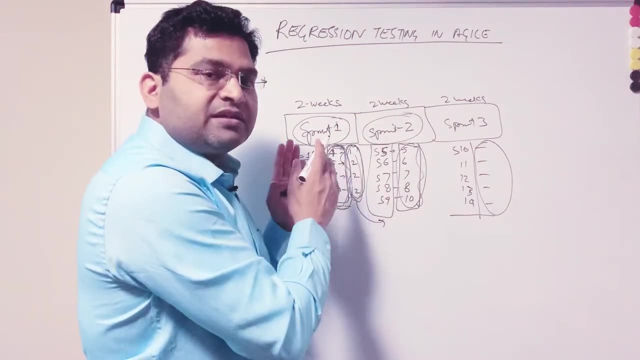 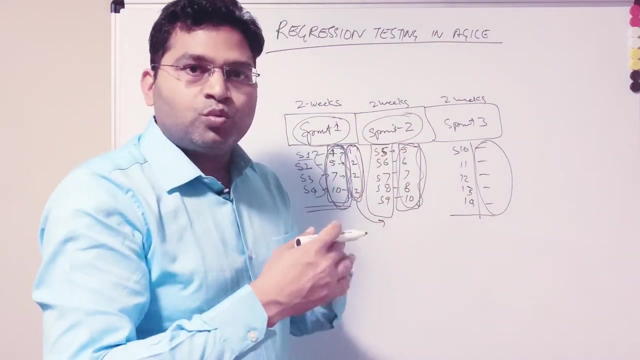 I'll have a team, or I have team members, who will automate these test cases so that when we are in the next sprint, we can basically, rather than executing these test cases manually as part of the regression testing, we will in sprint to run these test cases with the automation tool.